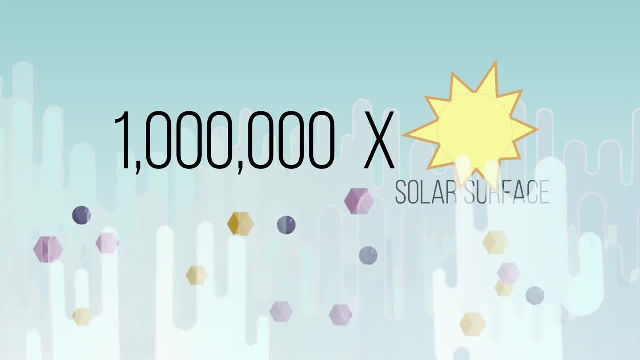 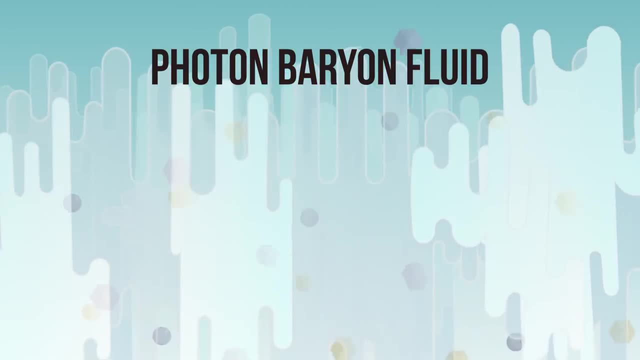 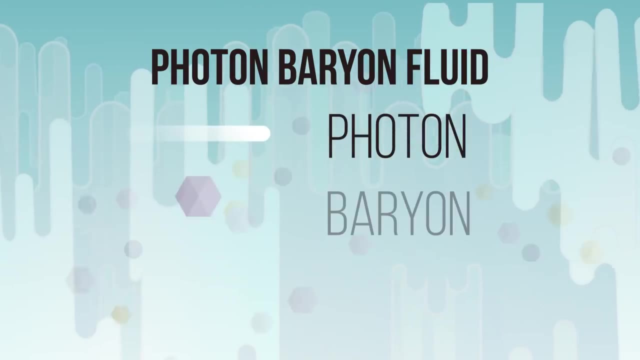 Celsius. That's roughly a million times hotter than the sun today, So hot that matter and energy are essentially the same thing. Our universe soup is called the photon baryon fluid because it's made of mostly photons and baryons with a dash of electrons. Photons are the 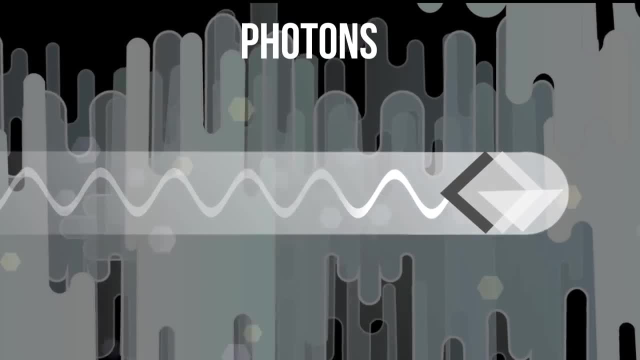 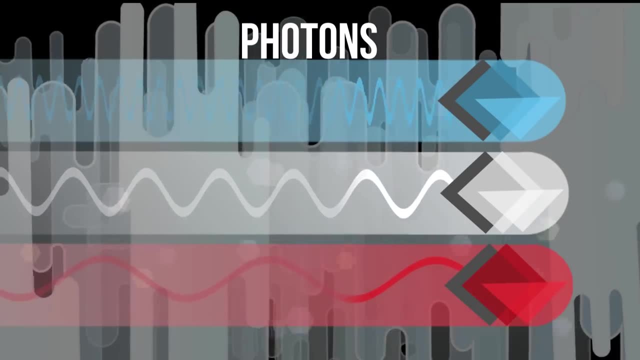 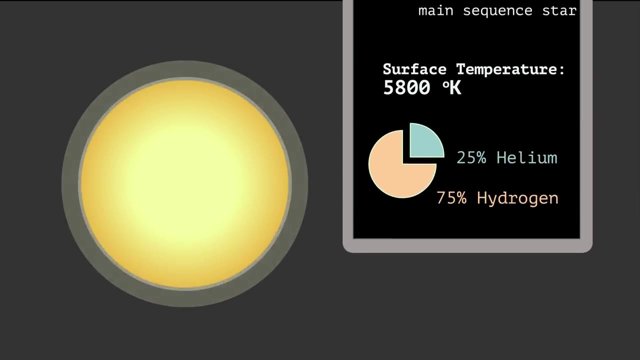 light particles, which carry the energy of radiation. They travel in the form of waves. Short wavelengths carry high energy. Long wavelengths carry less energy. When a photon is radiated away, it retains information about the source, such as its temperature, direction and even its chemical 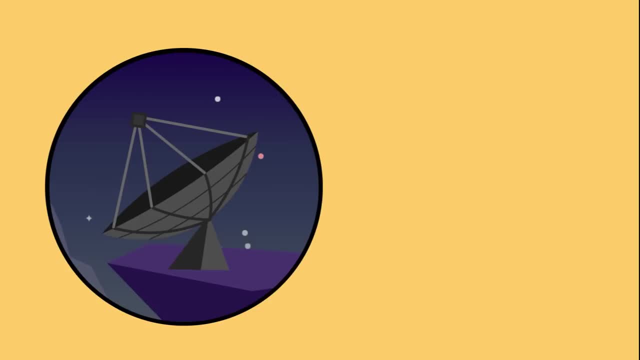 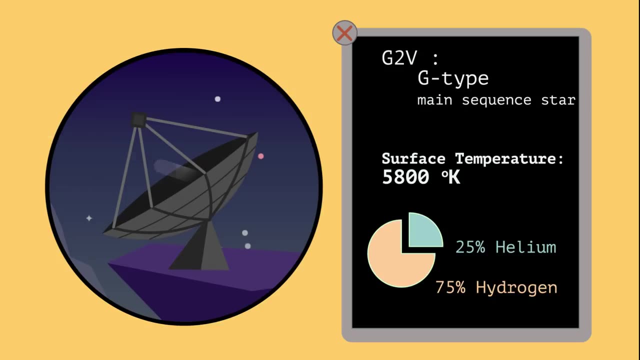 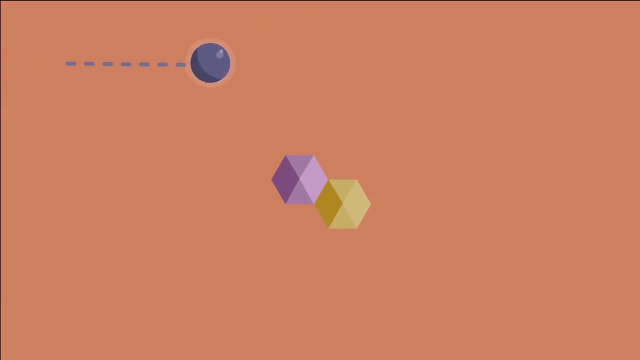 composition. They carry this information until they interact with matter, which means that the photons we detect today provide us with the history of their origins. Baryons include protons and neutrons, which make up the nucleus of the atom. The atom is the fundamental building block for all matter. 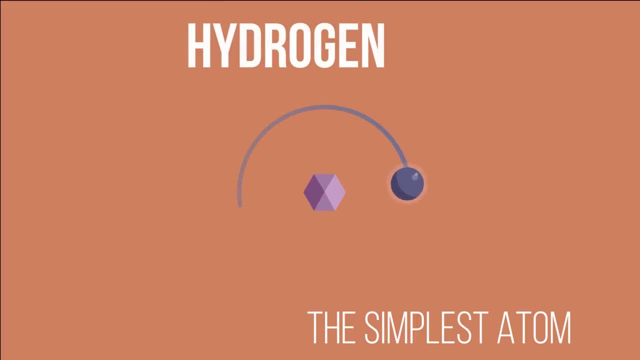 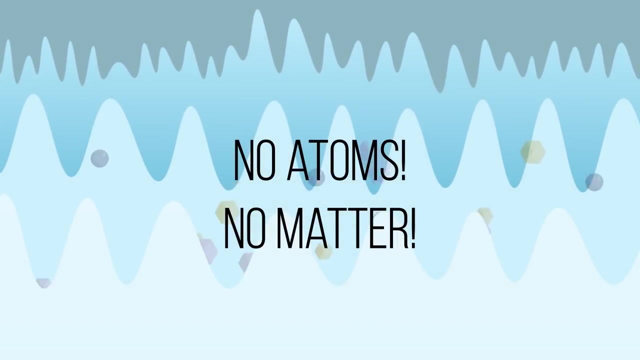 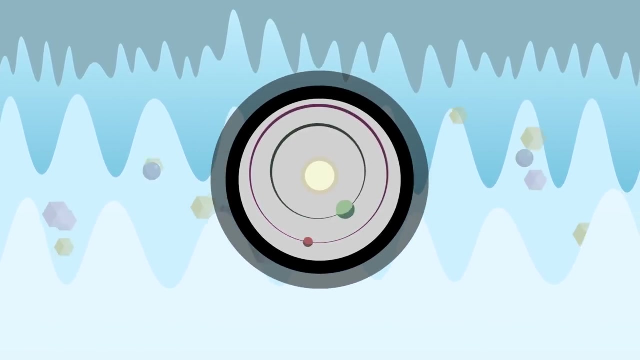 The simplest atom, hydrogen, requires one electron orbiting a single proton. but because the cosmos is so small and hot, the photons are energetic enough to blast electrons out of orbit. Thus no atoms are formed and nothing matters. The universe pretty much stays as this hot cosmic soup for a while. so let's fast forward. 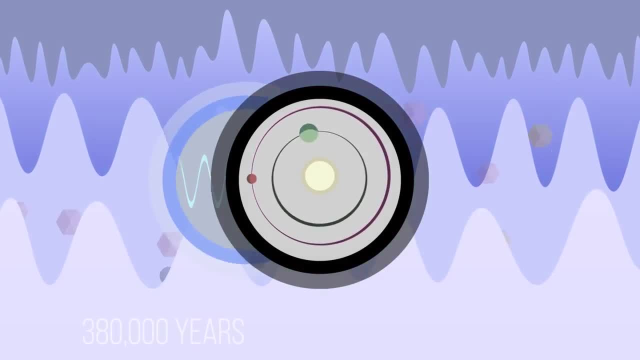 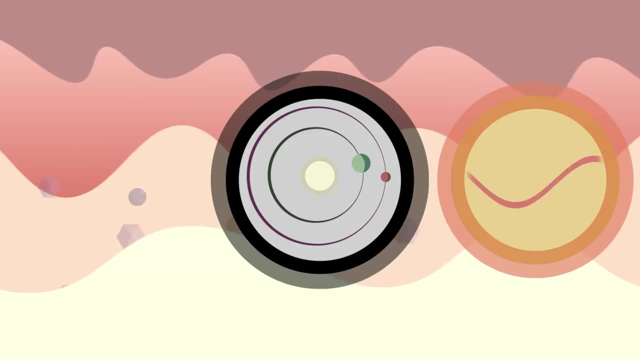 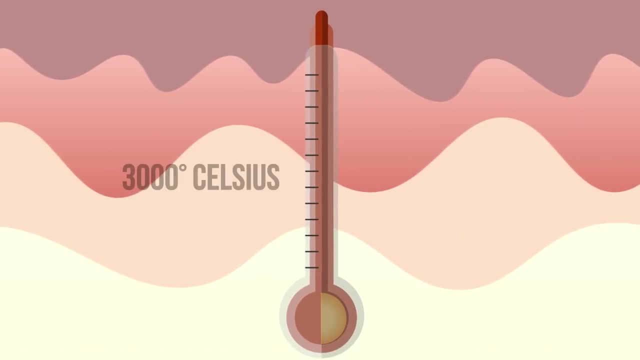 It is now 380,000 years later. As the universe expands, it stretches the wavelength of photons, resulting in a distribution of energy across space. The dispersion of this energy has caused the cosmic soup to cool to about 3,000 degrees Celsius, roughly half the temperature of the sun today. 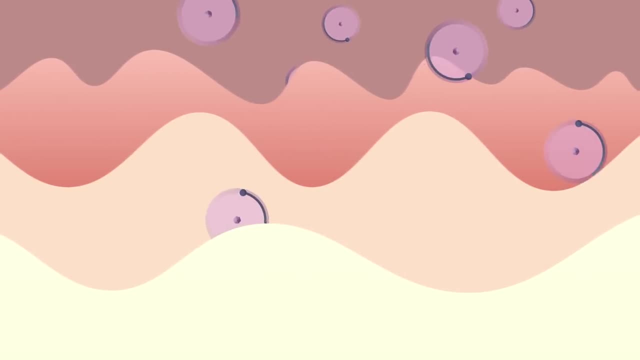 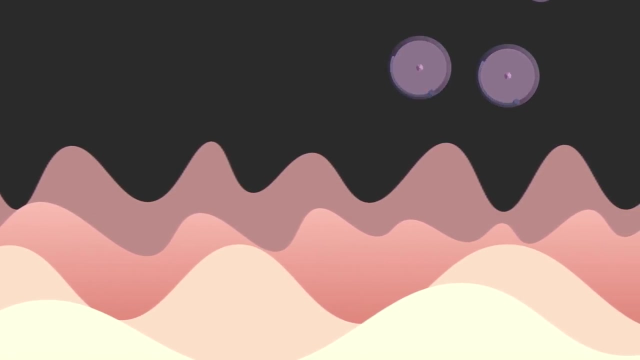 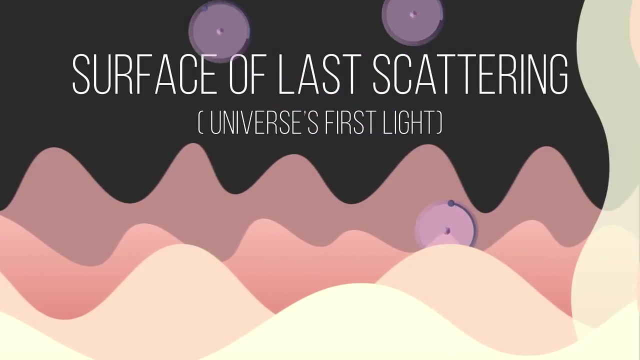 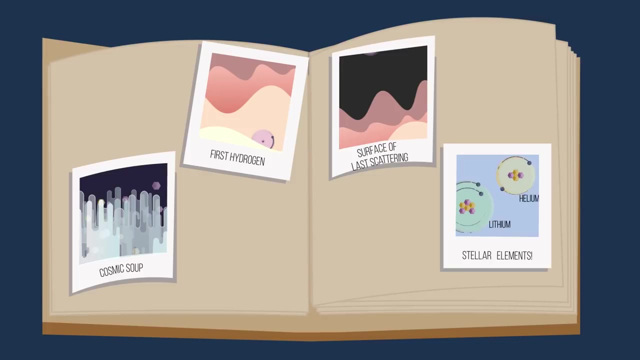 Since the photons are traveling with longer wavelengths, they are not energetic enough to scatter off electrons in orbit. The photon baryon fluid has evaporated. Let there be light And matter. This instant is recognized as the surface of last scattering The first light of the cosmos, a snapshot of the young universe. 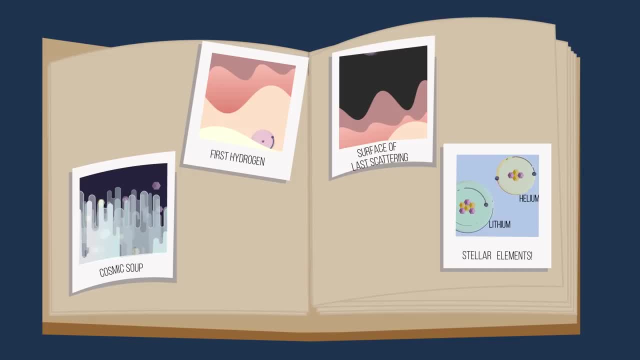 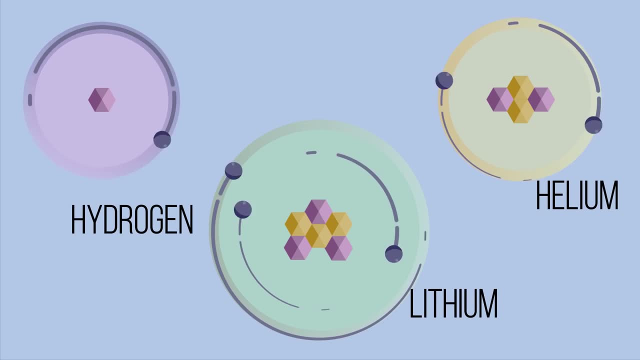 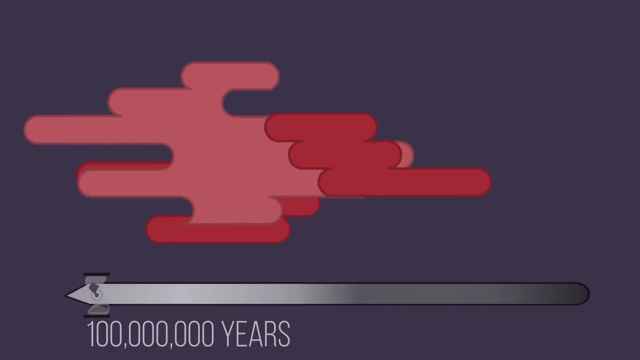 Photons can now move much longer distances and carry the information about this time further. Electrons are free to orbit baryonic nuclei, forming the basic blocks of all life. As we move forward in time, the photon wavelength continues to stretch At 100 million years. matter condenses to form stars. 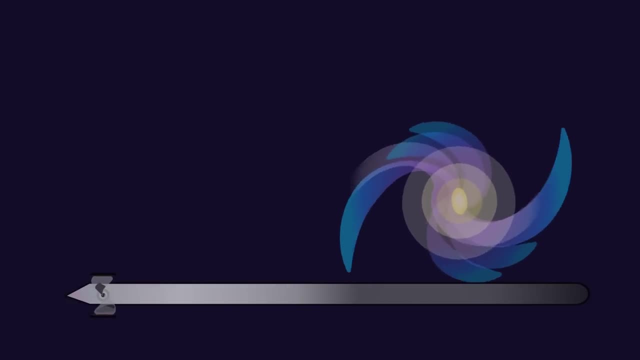 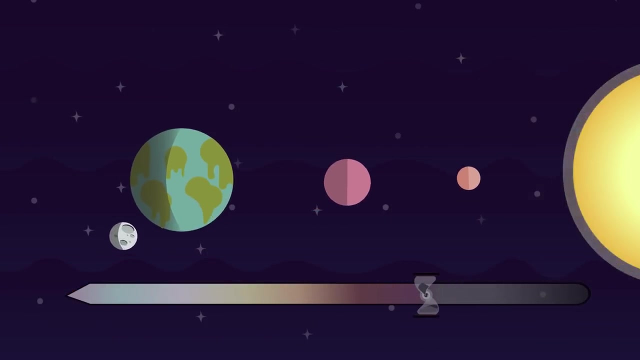 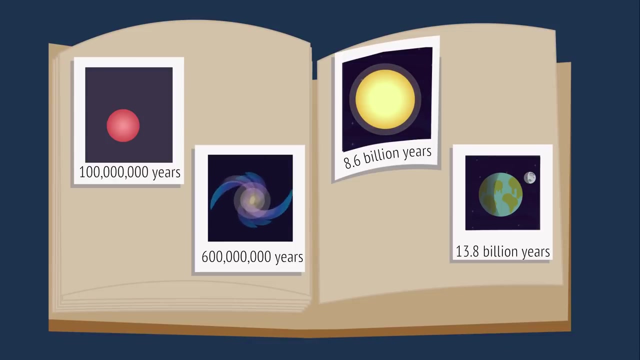 At 600 million years. our home galaxy, the Milky Way, is born At 8.6 billion years. the sun forms, giving birth to our solar system. Today, the universe is 13.8 billion years old. It has continued to expand and the photons of the early cosmos have continued to stretch. 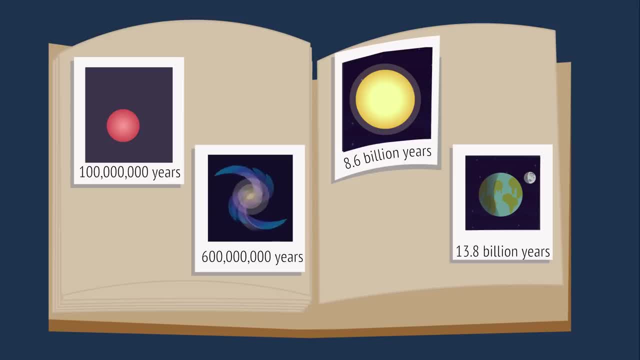 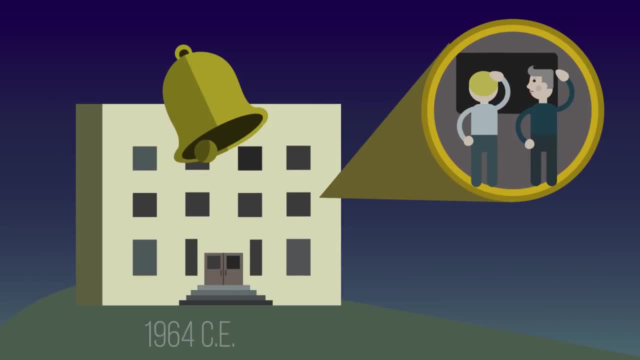 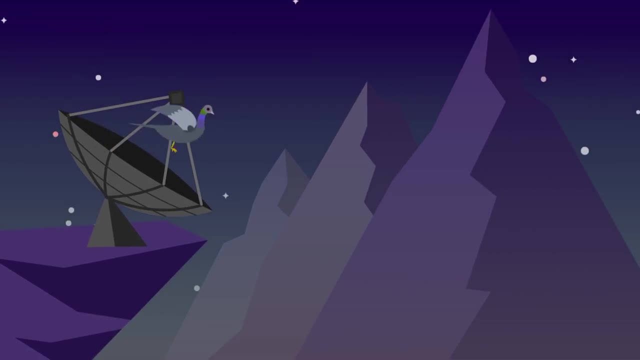 becoming invisible: low-energy microwaves, which are nearly radio waves. In the year 1964, two scientists at Bell Labs detect this radiation as noise in their radio telescope After cleaning up the white dielectric material they think is interfering with their data. 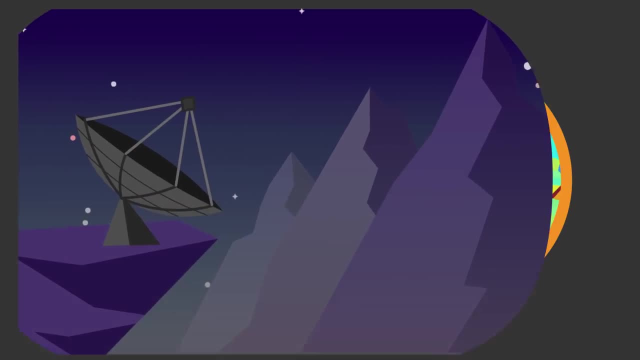 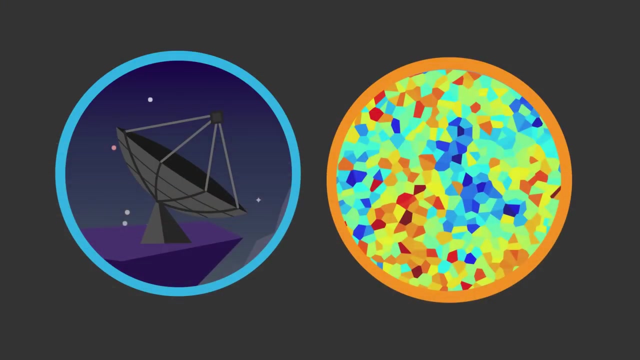 They discover this cosmic radiation is constant from every direction in the sky. After a paper publication, this apparent noise from the sky is recognized as remnant radiation from the earliest observable moment in the universe. This is the first time we've seen this. This is the first time we've seen this. 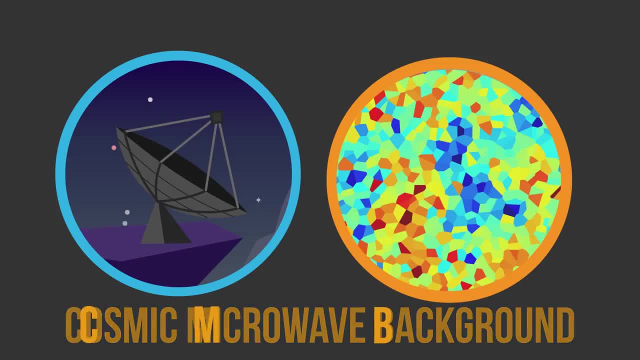 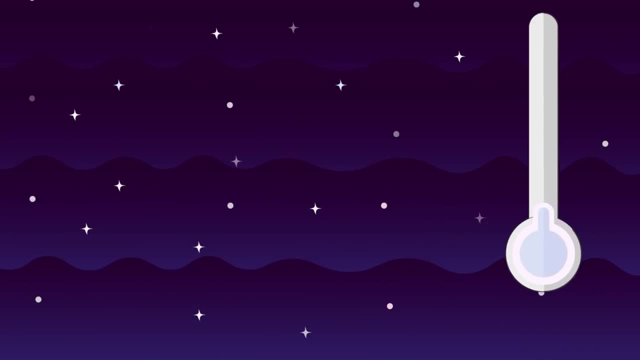 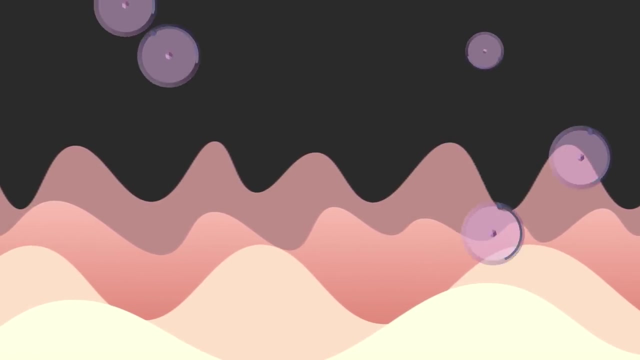 This is a baby picture of the cosmos called the Cosmic Microwave Background. This radiation from the CMB is what heats the empty voids of space to 3 degrees above absolute zero. Today we know the CMB is the heat radiation from the evaporation of the early cosmic soup. 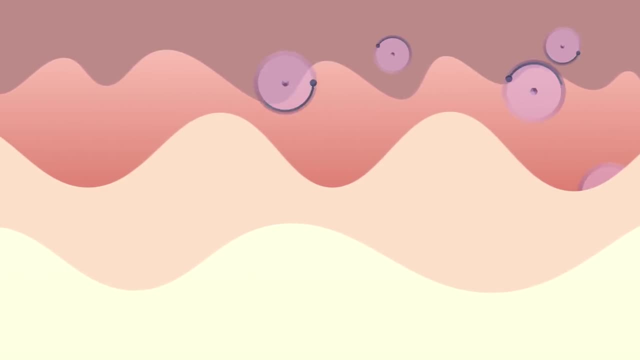 It is evidence that the universe was created by the CMB. It is evidence that the universe was created by the CMB. It is evidence that the universe was created by the CMB. The CMB is once a hot, dense fluid that has been expanding. 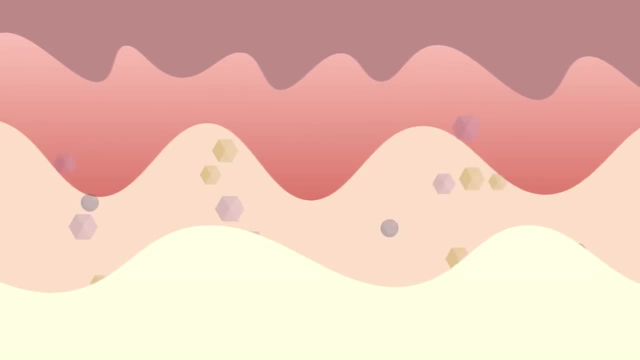 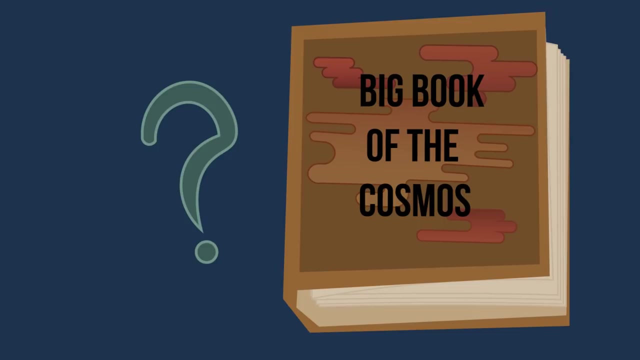 We interpret this as evidence of the Big Bang, but we don't know what happened before this picture. Cosmologists consider a number of origins for the cosmos based on this CMB radiation, But the most widely accepted model is the hot Big Bang. 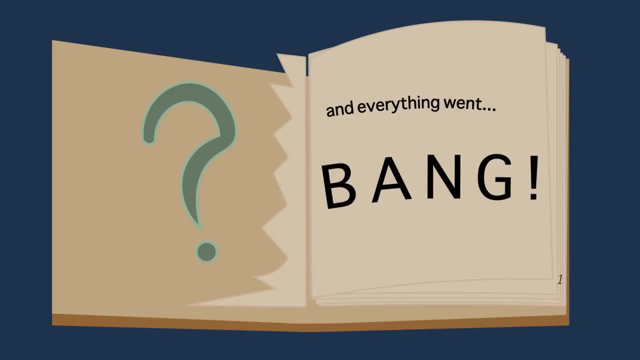 If the universe weren't expanding, we wouldn't be here and it would still be a hot soup of energy and matter you.